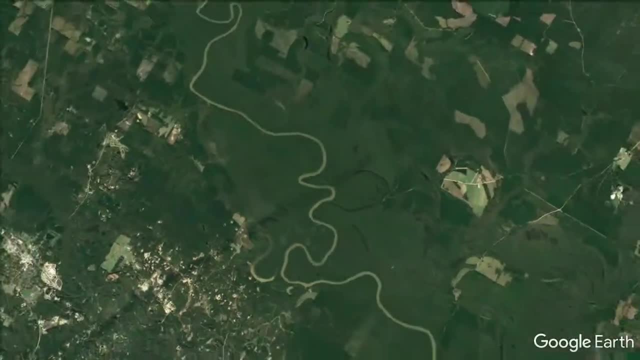 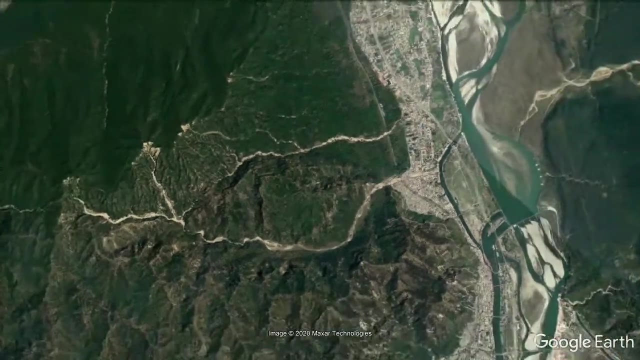 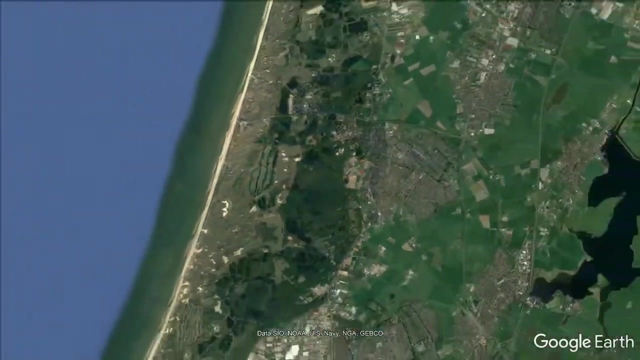 Within the ever-changing world, untouched wilderness keeps shrinking to smaller and smaller fragments. The small, fragmented patches cannot guarantee the survival of all species of the planet. We are running into a size problem, and this is especially apparent for larger species. Many larger species require considerable amounts of space. 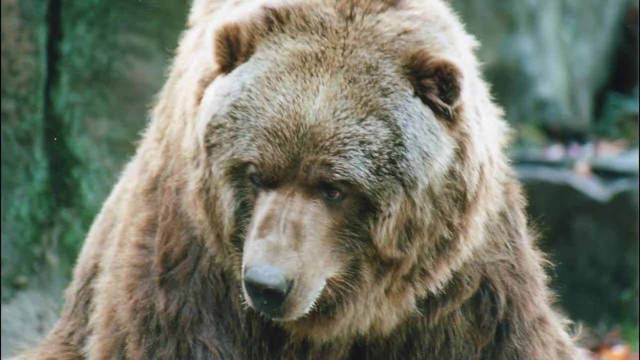 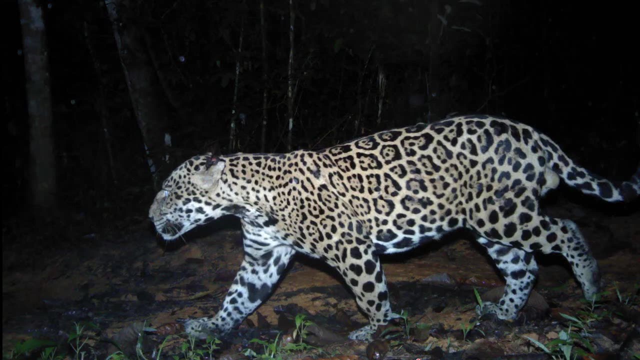 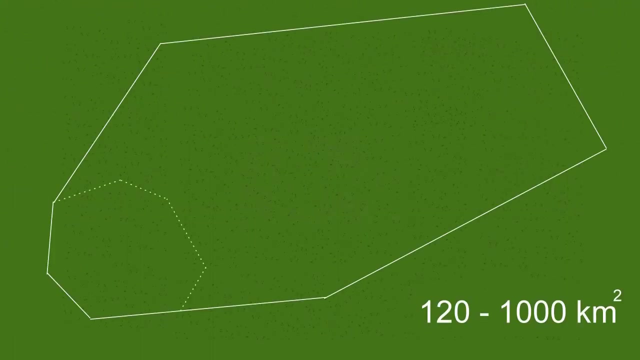 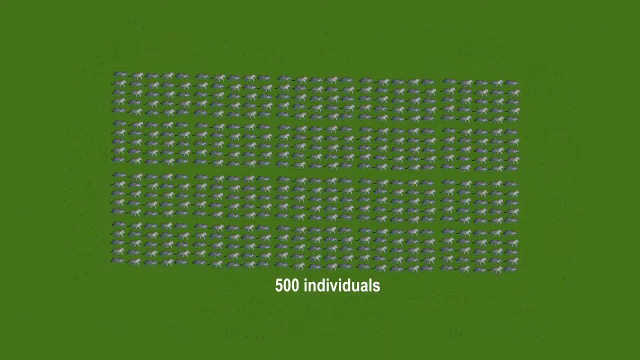 to sustain individuals. We will look at space use for large carnivores as an especially problematic group, using big cats as an example model. Here we will assess the intricacies and issues of space requirements and needs for these charismatic carnivores. Mathematical models have shown that it requires a minimum of 500 individuals within a single. 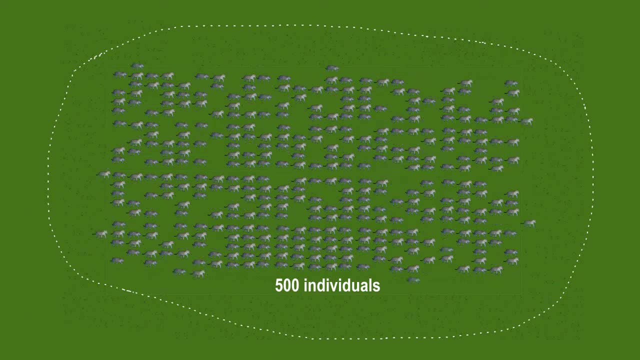 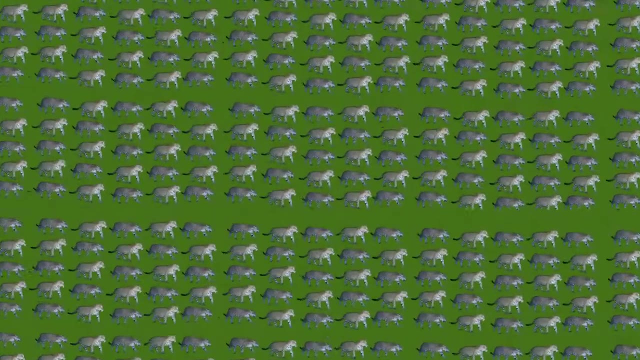 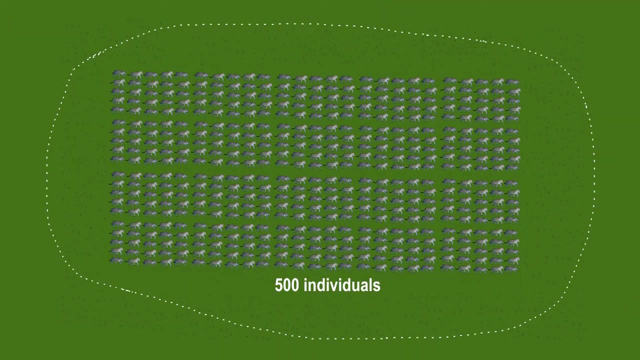 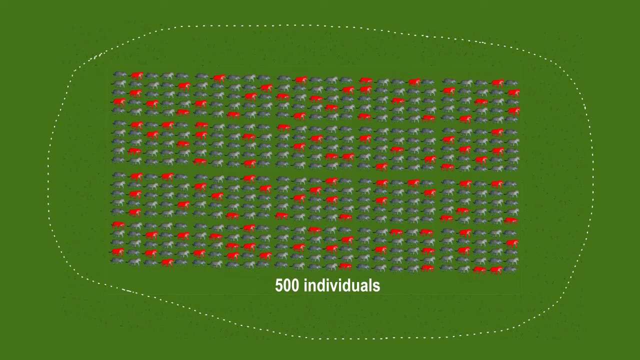 connected system to assure a high probability of survival for the total survival of all species of the planet. This means that all individuals should have the possibility to interact and mate. The 500 individuals assure sustaining of genetic variation and buffer against unfortunate chance events, For example, high selection against specific genes through disease or chance events. 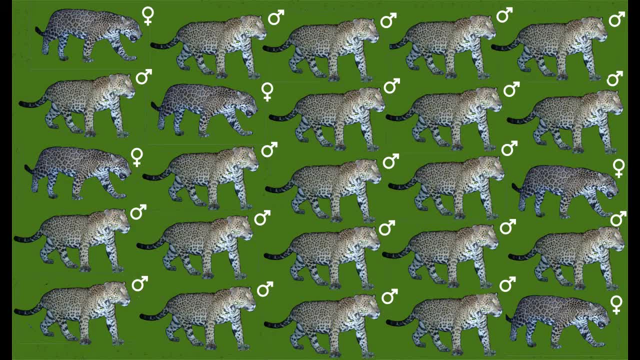 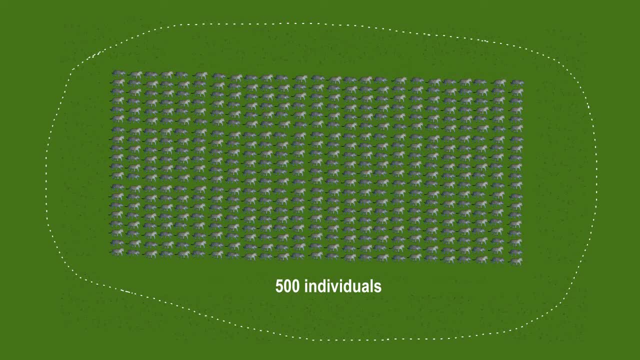 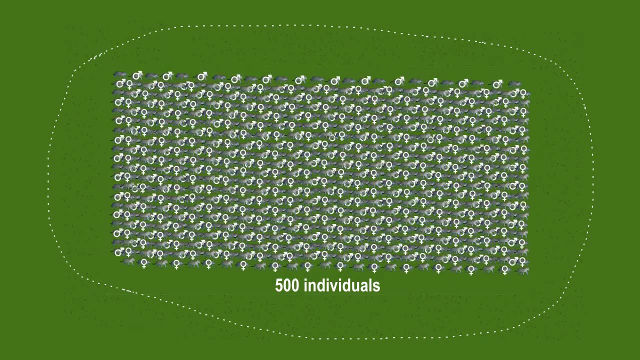 of higher than expected proportion of males being born at a certain time. It is therefore that we have to assure viable conglomerates of a minimum of 500 individuals, 250 adult males and 250 adult females, all being able to mate with each other- The easiest way to assure survival of a well. 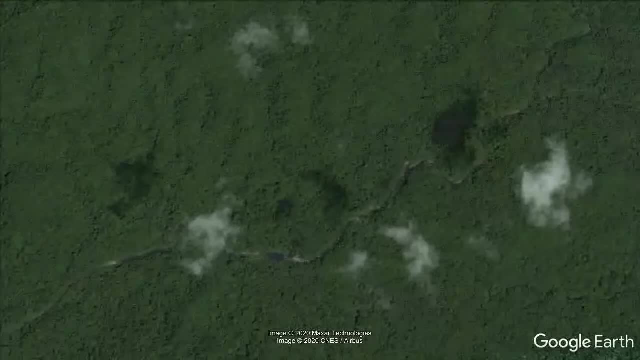 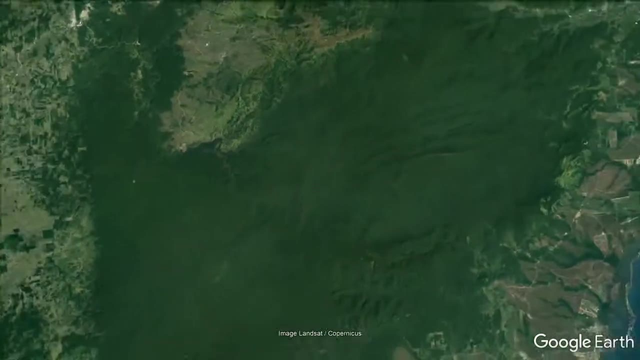 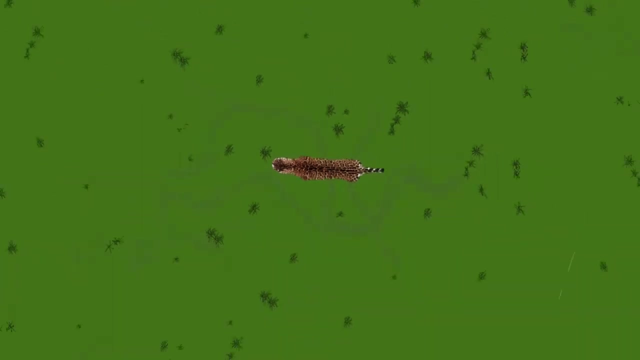 connected conglomerate of 500 individuals would be within a single wilderness landscape. The number of big cats that an area can sustain the carrying capacity depends on the amount of space that the individual needs. The home range of a single individual is dictated by the ability to acquire. 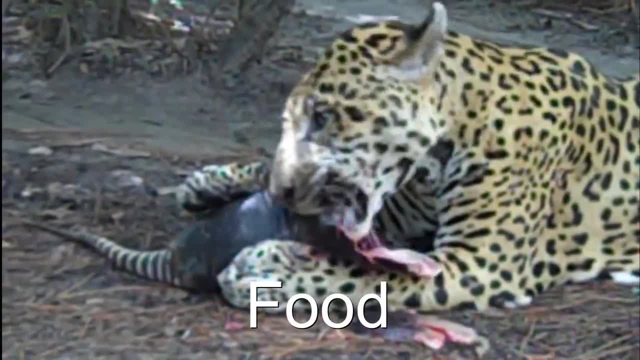 their primary resources: Water, food, shelter, mates. The distribution of these resources is dictated by the environment.